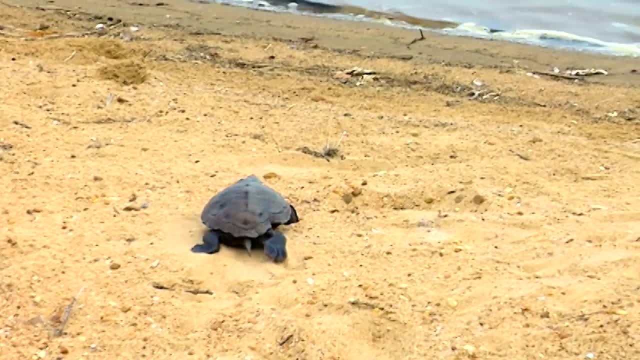 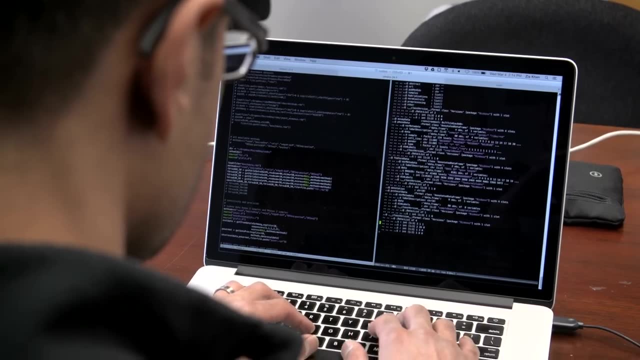 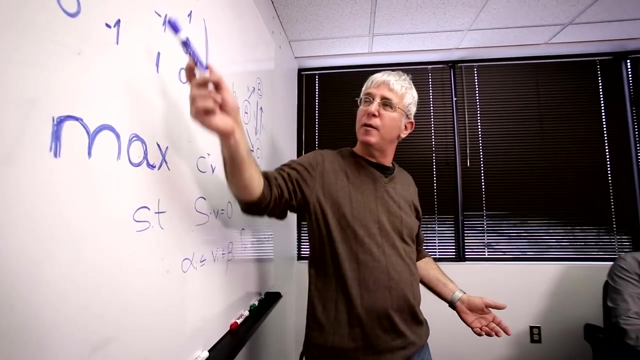 a new understanding of how living beings interact. The Center for Bioinformatics and Computational Biology, known as CBCV, brings together researchers from computer science, molecular biology, genomics, genetics, mathematics, statistics and physics Together. they are combining big data and biology. 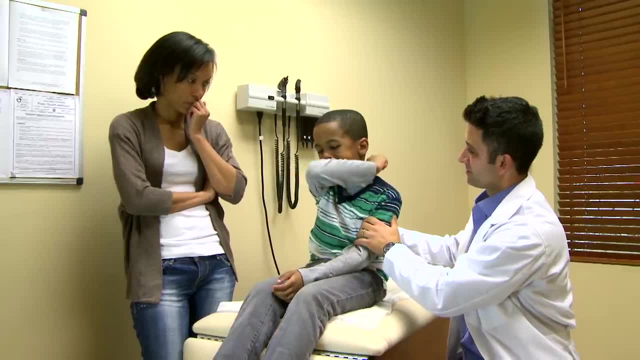 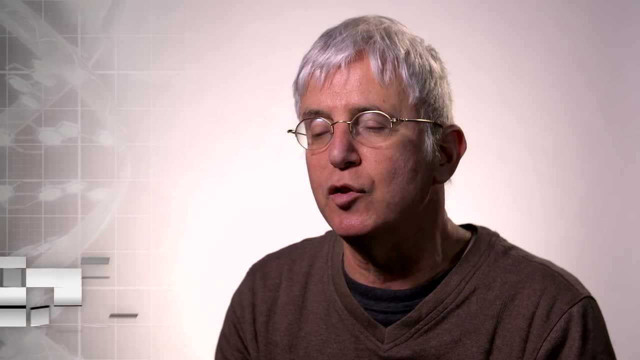 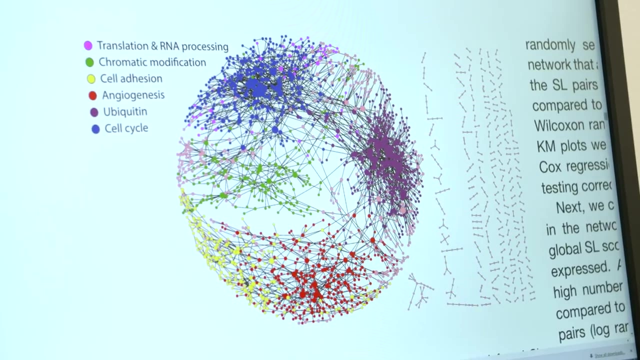 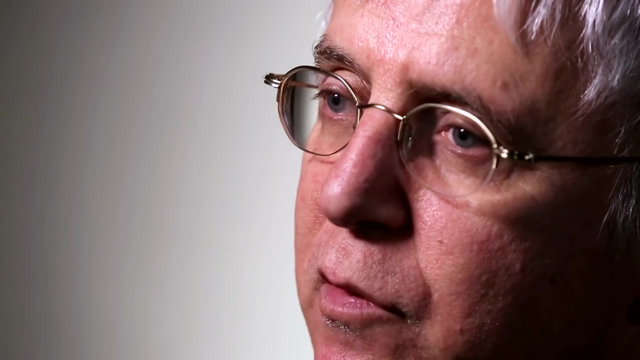 To better treat disease, promote healthier lives and understand how the world around us has evolved. The mission is to try and make sense of these huge amounts of data that are now generated in biomedical research and apply the most cutting edge quantitative analysis approaches that we have to interpret this data into meaningful insights and results. 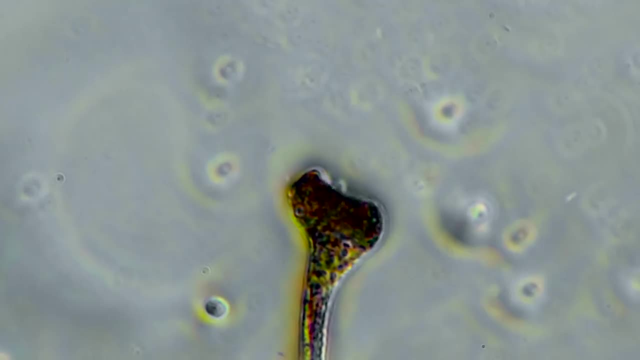 Whether it's cholera in Haiti, intestinal parasites in Africa or the spread of COVID-19,, the University of Maryland is committed to improving the health and well-being of our students. The Center for Bioinformatics and Computational Biology, known as CBCV, brings together researchers. 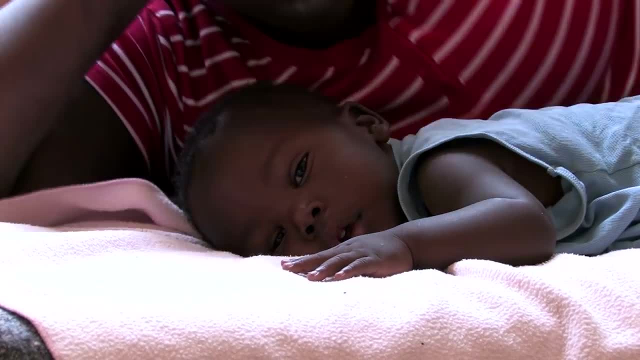 researchers and researchers from around the world to help develop new approaches to the health and well-being of our students. The Center for Bioinformatics and Computational Biology, known as CBCV, brings together researchers from around the world to help develop new approaches to the health and well-being of 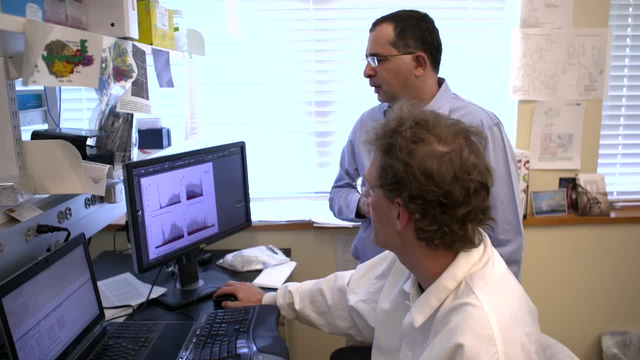 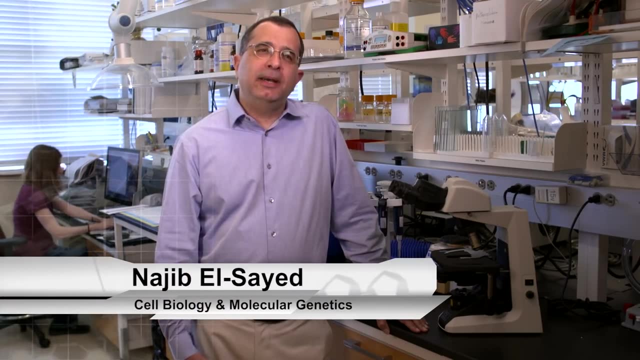 our students. Whether it's cholera in Africa or bacteria that can make children in developing countries gravely ill, researchers in CBCV are using the power of computational biology to identify causes and offer solutions. My lab focuses on combining computational approaches with wet bench experimentation. 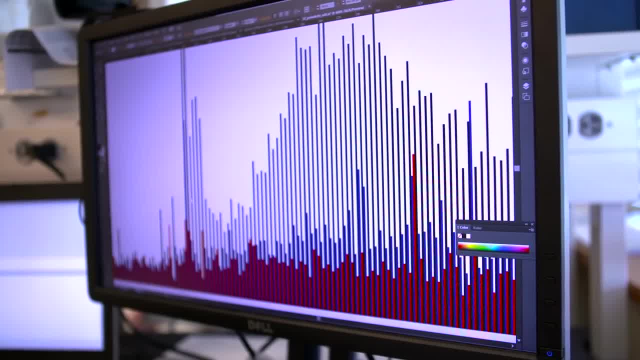 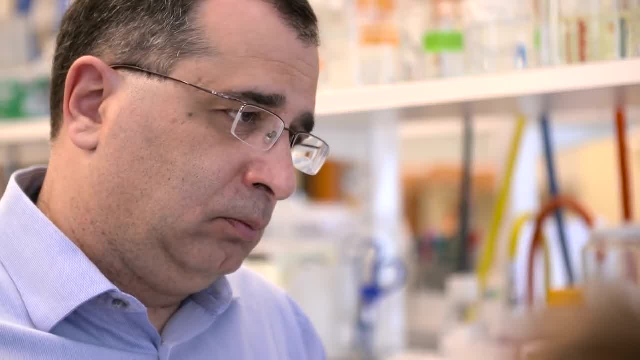 Essentially, what we do is we collect and analyze large amounts of genetic data from the pathogens that infect human beings, on which genes they turn on and they turn off as they infect the human host. We collect data on the genes that the human host turns on and turns off in response to. 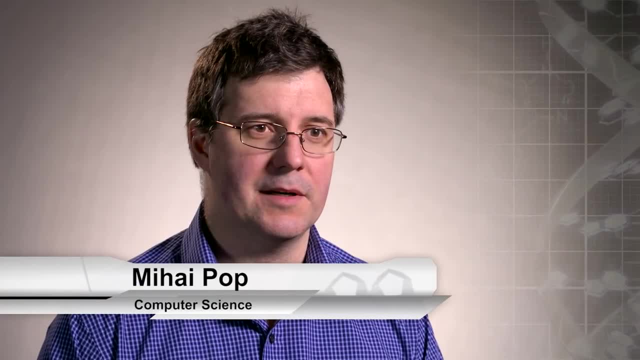 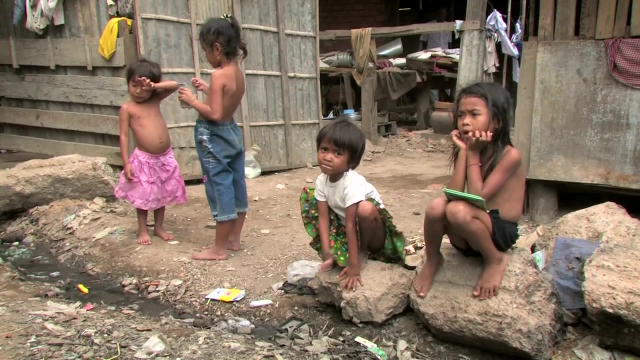 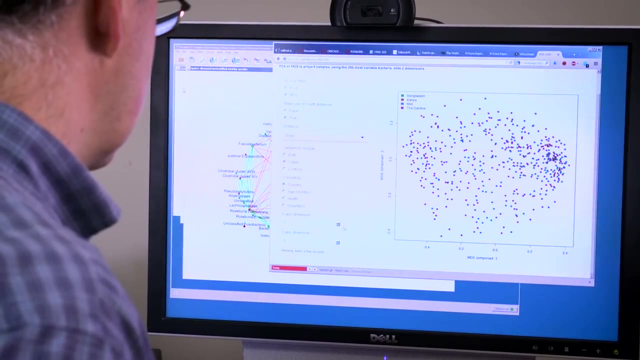 the infection. One of the big projects we have in our lab has been the study of diarrhea in children in developing countries. More children die of diarrhea in these countries than HIV, measles and malaria combined. We are developing new computational techniques that allow us to decide which of these bacteria. 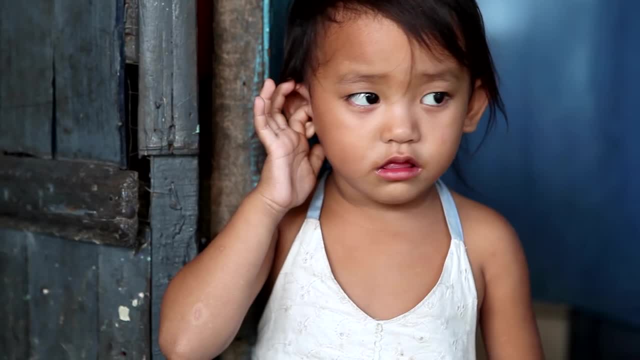 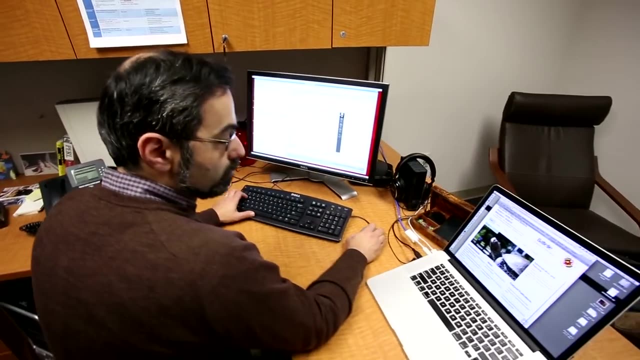 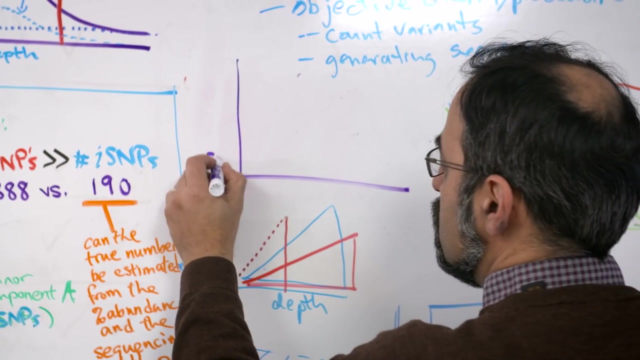 might possibly cause diarrhea or which of these bacteria might protect the children against diarrhea. CBCV is part of a multi-institutional study focused on regulatory science for tobacco. We are providing expertise in big data management and biostatistics to better understand the 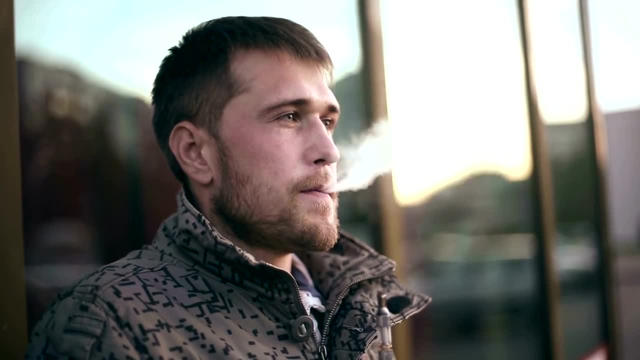 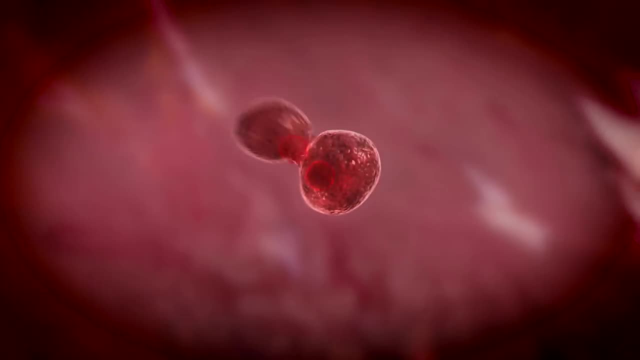 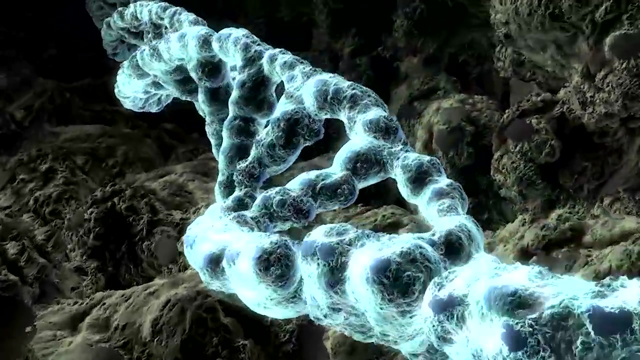 physical and psychological effects of new products like e-cigarettes. We are also using high throughput genomic sequencing to glean new knowledge on how organisms develop. My group will be focused on the evolution of a folding structure that forms in the fruit fly. We'll be studying its evolutionary past in a lineage of flies and we'll be studying 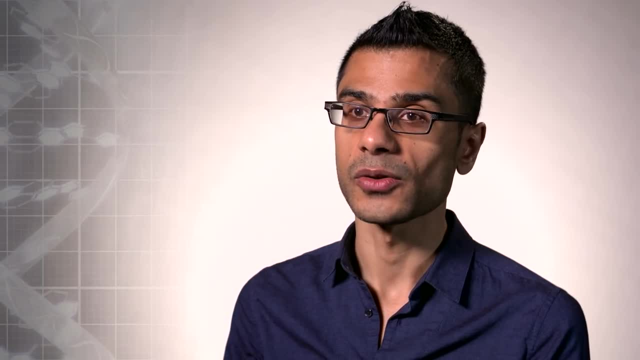 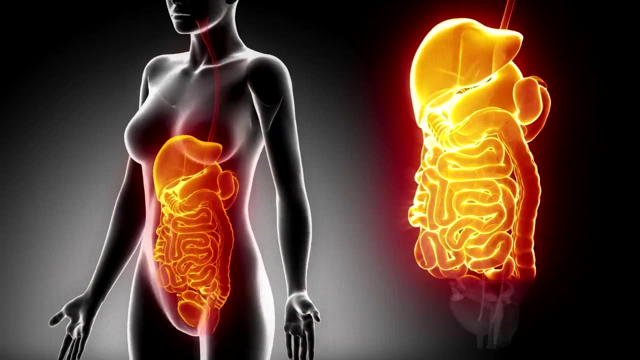 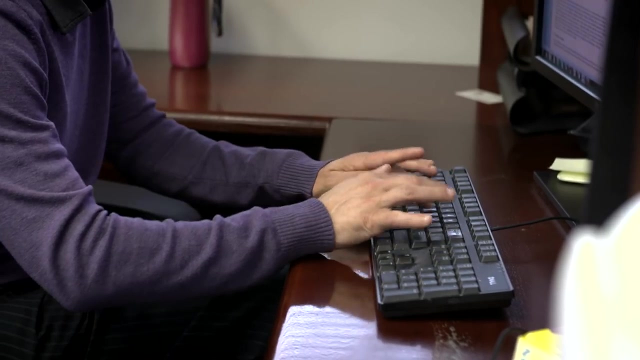 its potential capacity for future evolution. A fundamental question in evolutionary biology is to understand how structures like organs and limbs actually evolved. This research will help us understand how that happened. Other faculty are looking at genetic changes in cells that can lead to cancer diabetes. 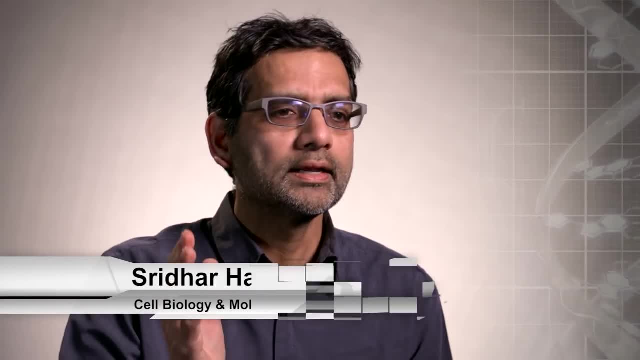 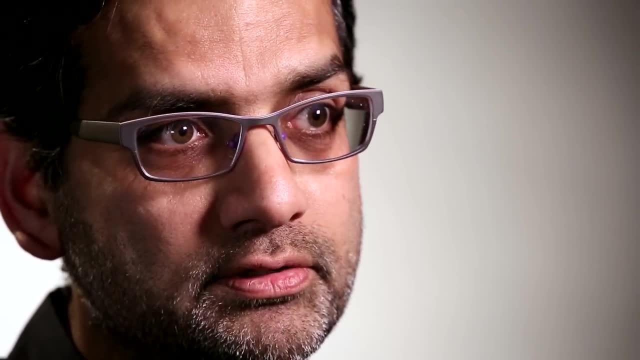 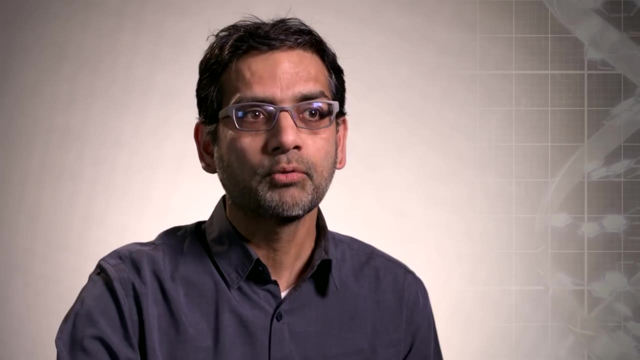 Parkinson's disease or Alzheimer's. The broad million dollar question in the field of biomedicine is: how does an individual's genome determine the person's susceptibility to different diseases? How do specific genes get turned on? Ultimately, everything hinges on that process as to what makes it manifest itself into a 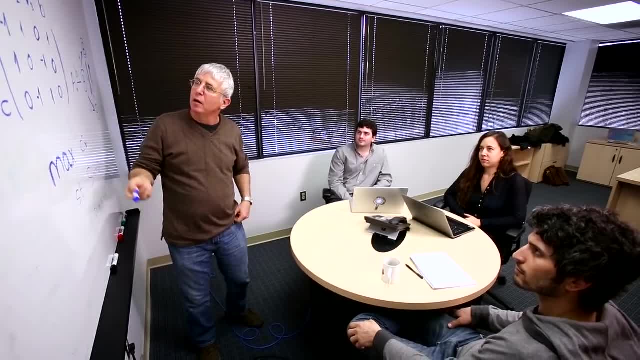 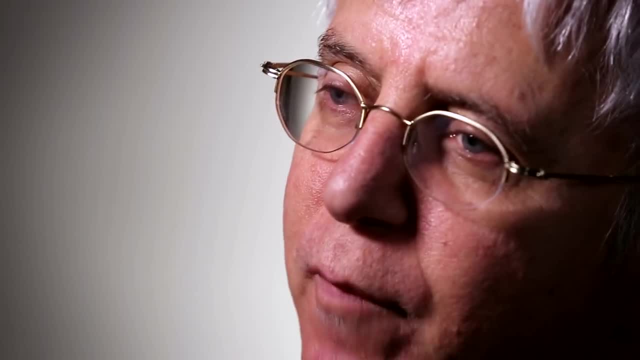 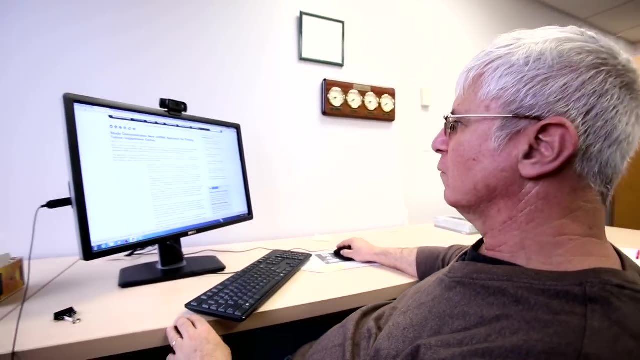 phenotype or a disease or what have you. CBCV is also using big data to identify genetic markers that can pinpoint new therapeutic treatments. The main driving force of my research these days is genetic markers. I'm focused on cancer and mainly on identifying new drug targets to treat cancer. 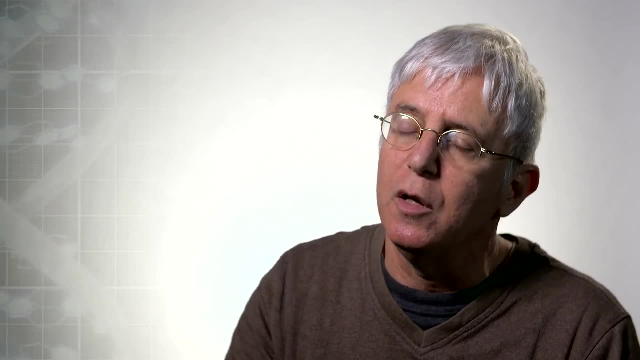 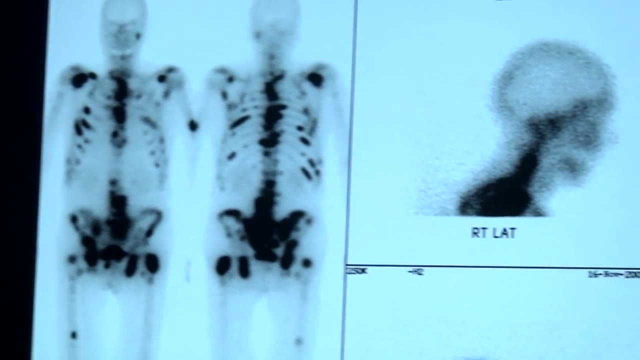 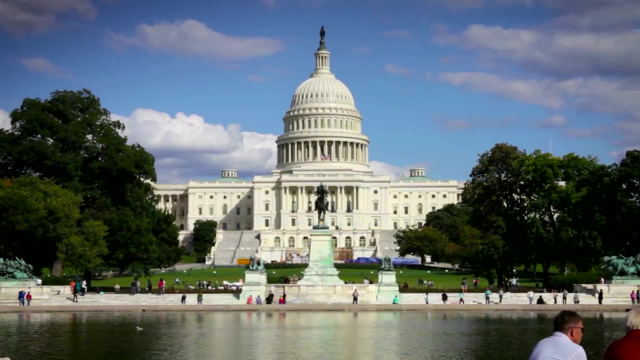 The main problem we have now with the development of new anti-cancer drugs is that there is tremendous success initially, but then, because cancer is heterogeneous and clonal resistant develops. The University of Maryland is located just outside of Washington DC, allowing CBCV. 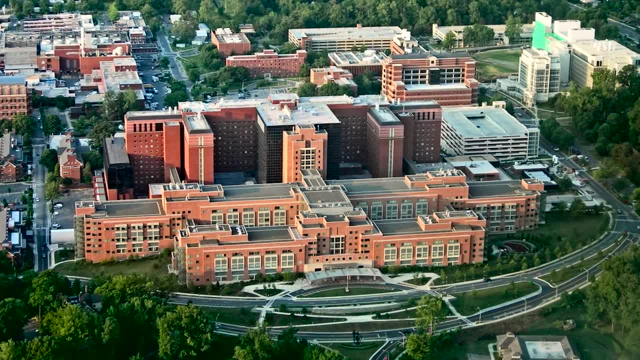 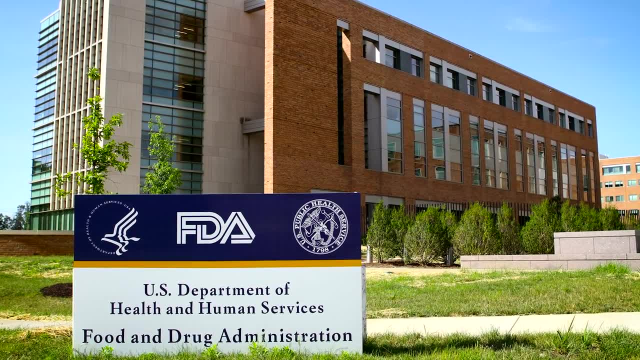 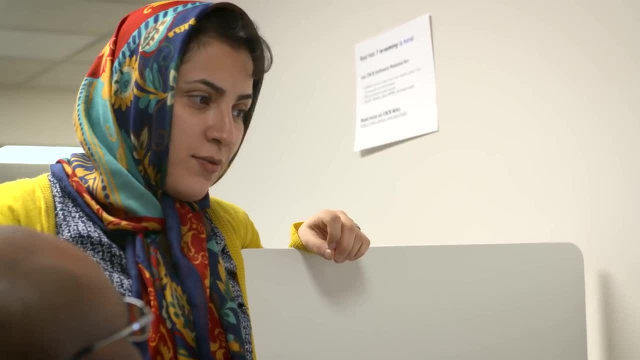 faculty and students to interact with scientists at the National Institutes of Health and its National Cancer Institute. Other research involves the US Food and Drug Administration and the University of Maryland School of Medicine. These partnerships are especially valuable to the Center's graduate students, who constantly 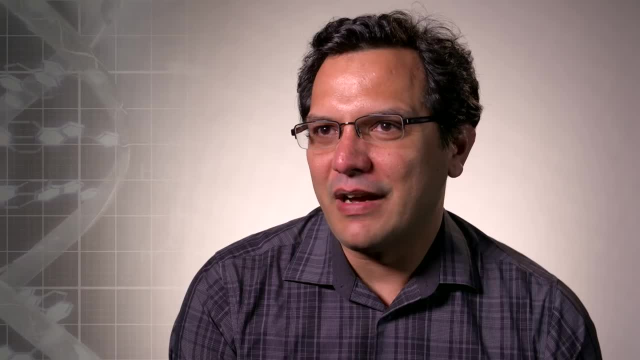 bring a wealth of new knowledge and new ideas to the table. I don't think any project is successful without a really keen, really intelligent graduate student driving it. For certain projects that we've been working on, we've been working on a number of projects-